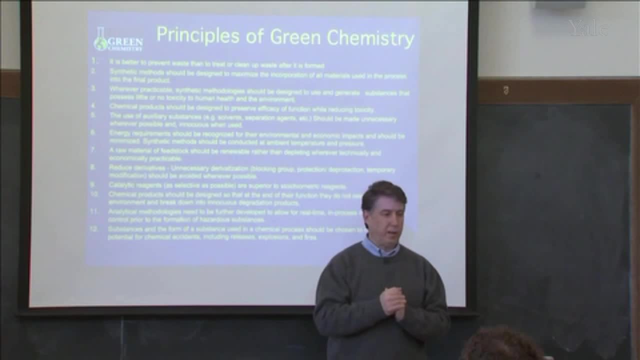 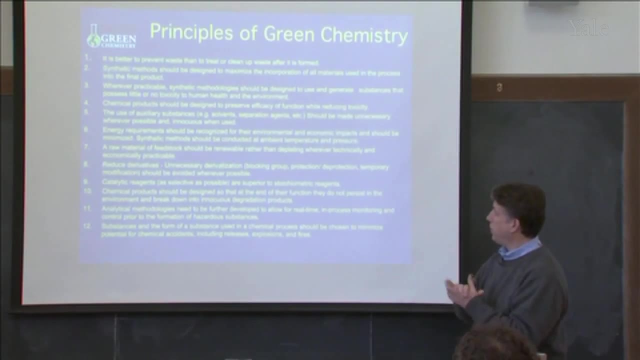 apart and put back together and to see if they have any utility or any value. And what is useful about these is that they've been around for coming on 20 years out there with lots of discussion, and they are at this point, widely used And we can talk a lot. 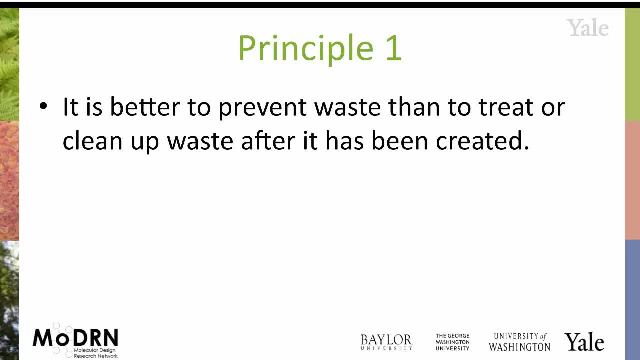 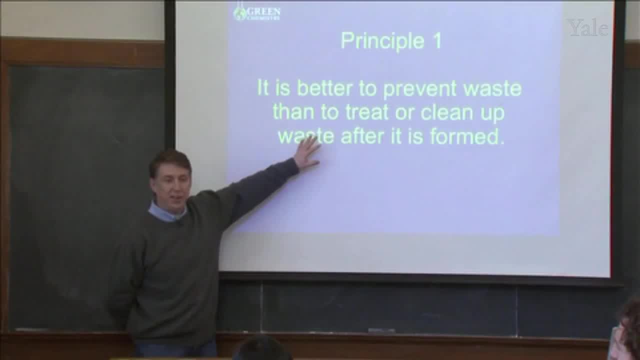 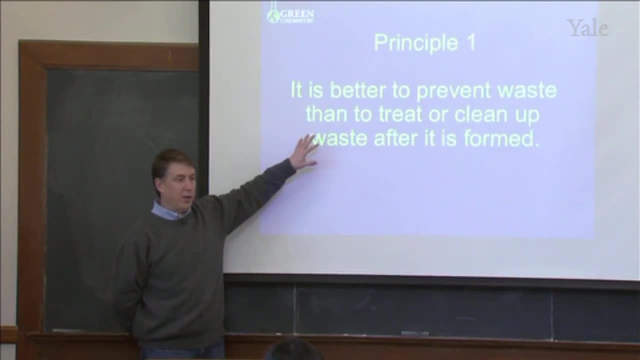 more about this, But let's talk about principle one. It's better to prevent waste than to treat or clean up waste after it's formed. So the reason that it's necessary to state this is because the entire history of environmental protection has been that you know, you just treat and control your waste and all's well. 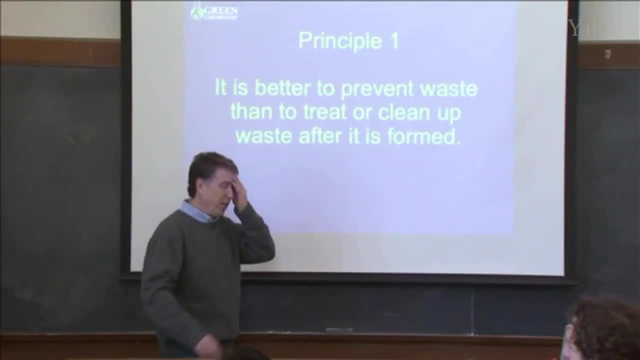 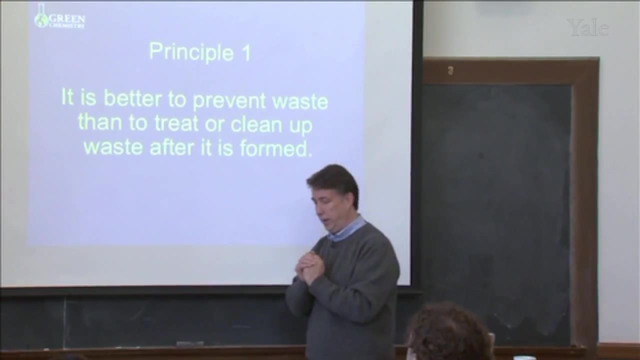 with the world. So that has been the whole. industries have sprouted up to clean up after wasteful manufacturing processes, wasteful end of life. But there's an inherent problem with the create and clean up waste issue, And one has to do with the loss of thermodynamics. 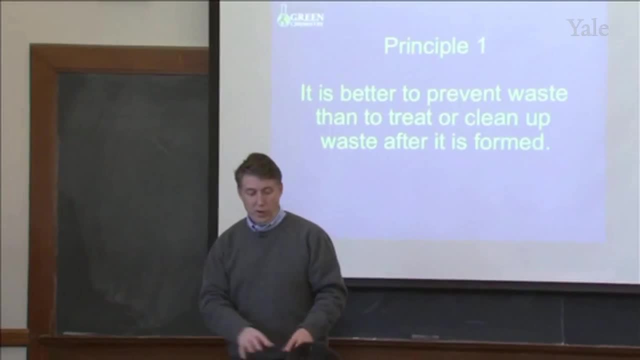 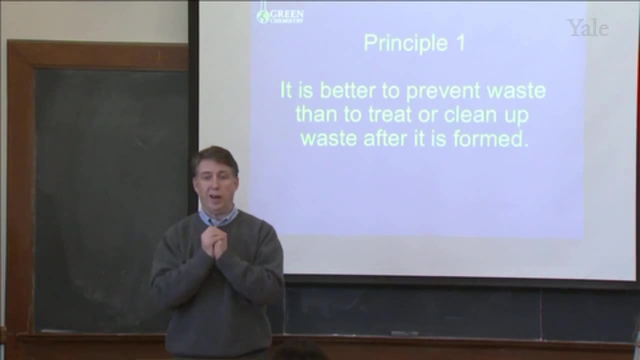 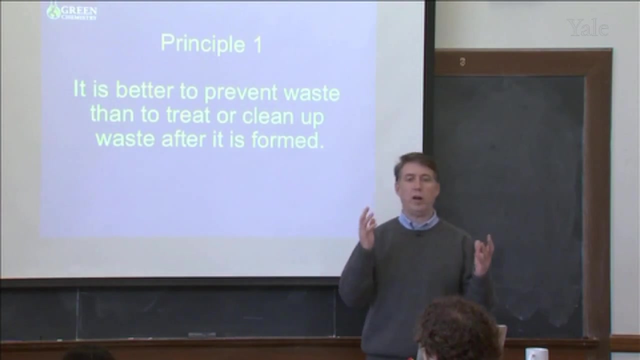 Okay, So we talk about. well, we'll make sure that if that we'll close our loops, there won't be any emissions, there won't be any exposure to people, workers, consumers. there won't be any exposure. There's no exposure to the air, to the water. These loops stay closed. based on thermodynamics. 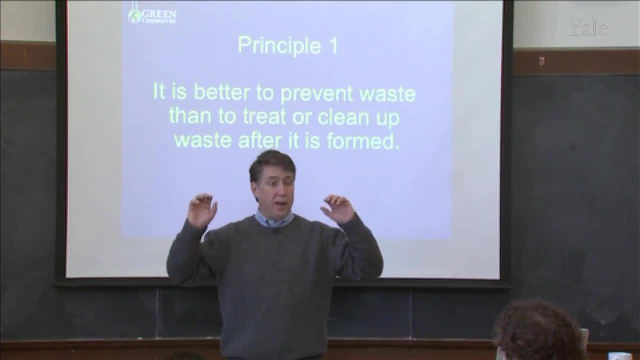 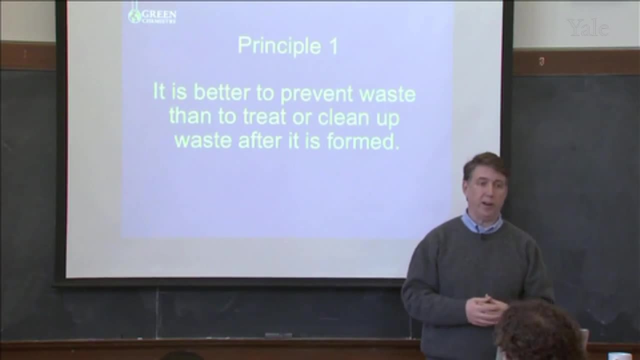 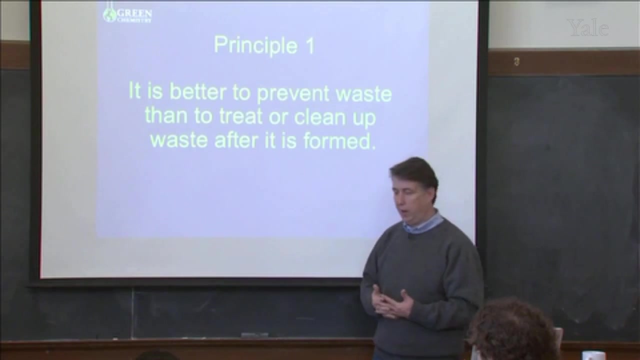 right up until they don't And they dissipate. And when we're talking about substances that persist, that bioaccumulate, that build up into our bodies and the biosphere, the idea of, well, it's okay, if we can create it, we'll just clean it up, becomes an experiment that 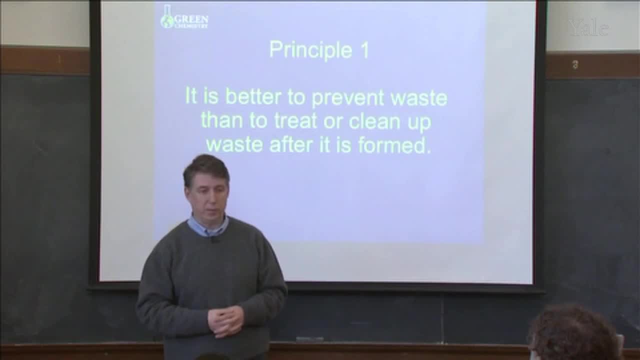 we've run for many, many decades and shown that it doesn't. It doesn't work And, of course, anything I say, please feel free to challenge. But the other issue is that: does it cost money to treat or clean up waste? Does it cost energy? 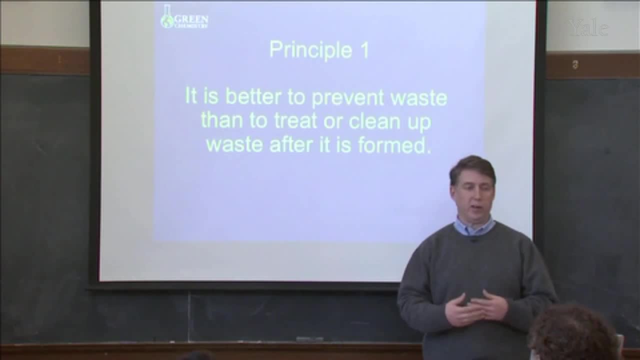 Do you have to expend energy to separate the waste, to clean it, to treat it? Does it add performance to a product? Does it add efficiency to a manufacturing scheme? Why have we thought that environmental issues cost a lot of money for decades? Because this has largely been. 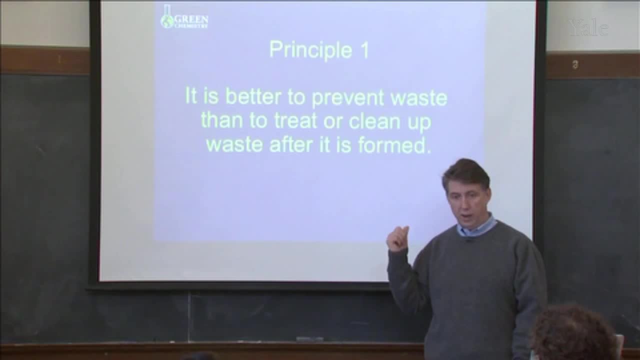 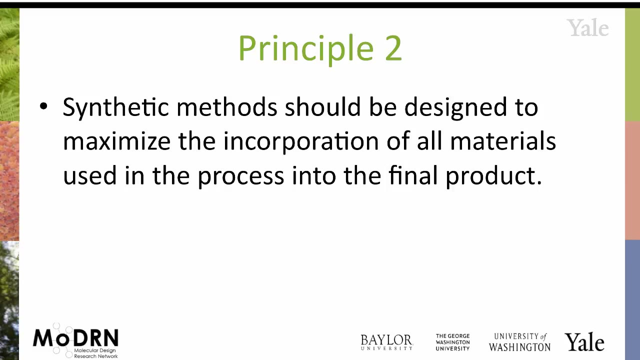 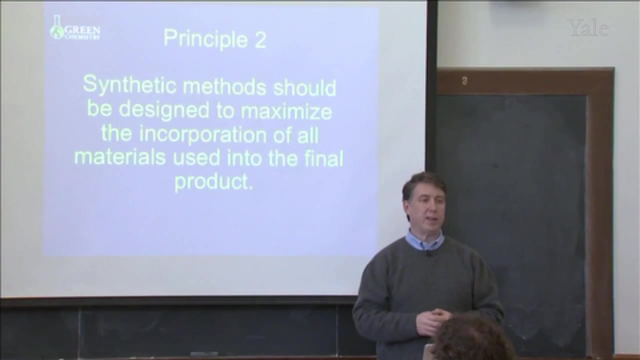 the approach that we've used. Our approach to dealing with these issues has largely meant that you were going to have a significant expenditure. Principle two: Synthetic methods should be designed to maximize the incorporation of all materials that are used into the final product. Basically, if you're going to put 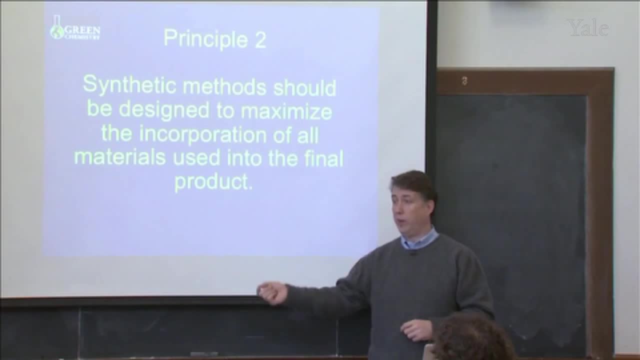 an atom in. you want it to wind up in your product and not into your body. That's the first principle. It's a concept called atom economy. We're going to talk a lot about it and we're going to be able to actually measure what's the atom economy of these transformations. 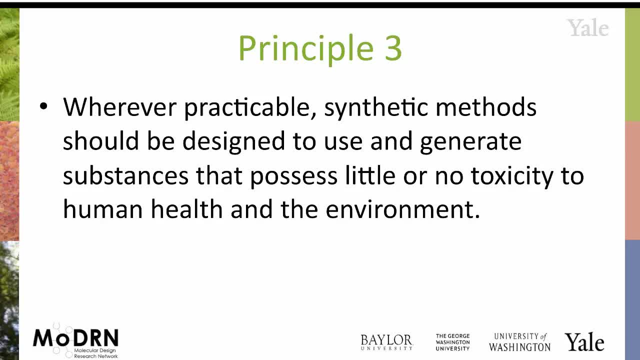 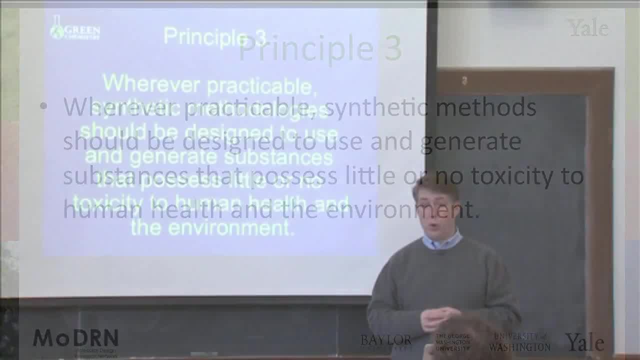 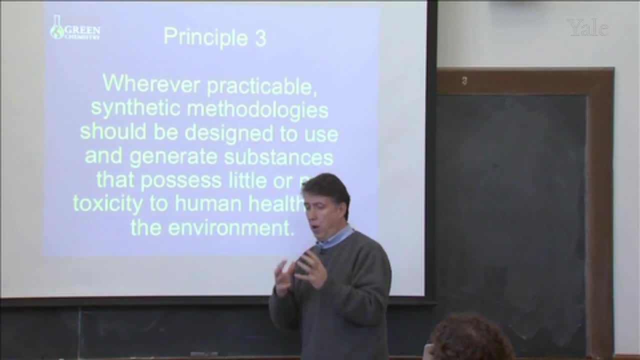 Principle three: Whatever practical synthetic methods should be designed to use and generate substances that possess little or no toxicity to human health and the environment. So we captured this, So you want to use, whether it's your reagents, your feedstocks and all. 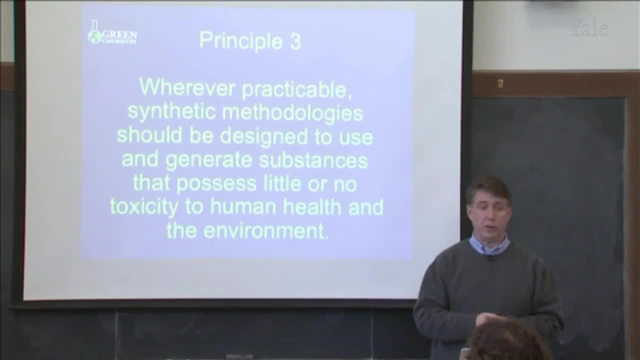 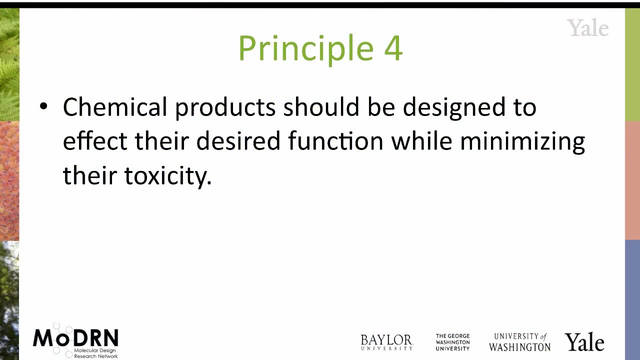 of these transformations. Principle four: Chemical products should be designed to preserve efficacy of function. So not that you have a very nice soap that doesn't have any toxicity, but it doesn't work as a soap. Preserve the efficacy of function while minimizing toxicity. 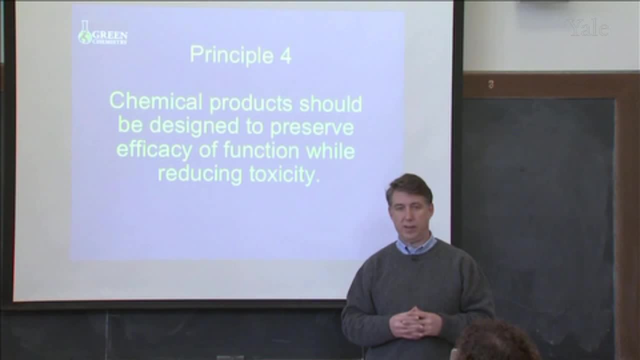 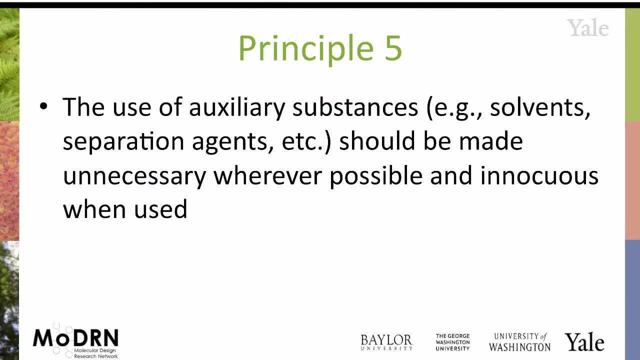 this is going to be a large section of this class. when we start talking about molecular design, we start talking about hazard reduction. this is what we're talking about: auxiliary substances. there's a whole lot of things that go into manufacturing. there are solvents, there are separation agents, there's 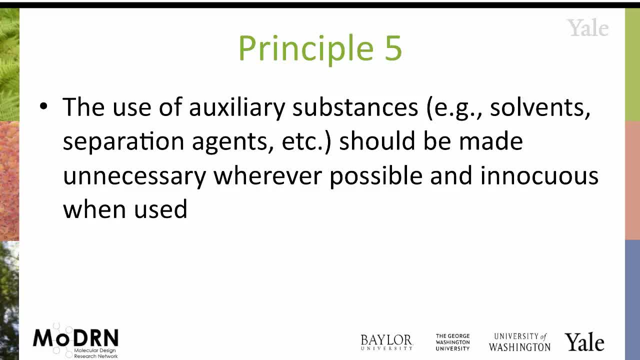 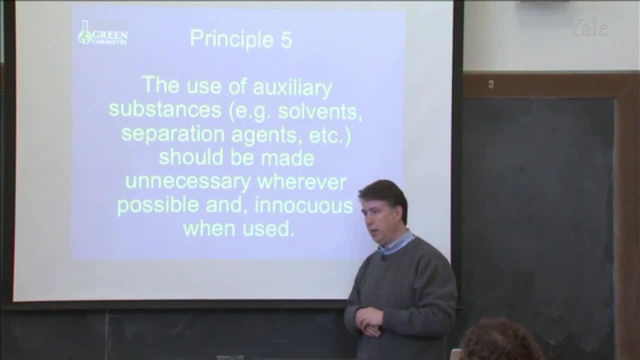 there's energy that's put in to to bring about separations that we'll talk a lot about, and these can make up a huge percentage of the waste stream- and pharmaceuticals- it's estimated that 80% of the waste are the solvents that are. 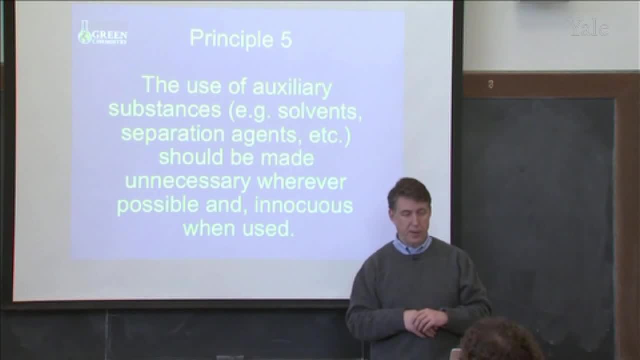 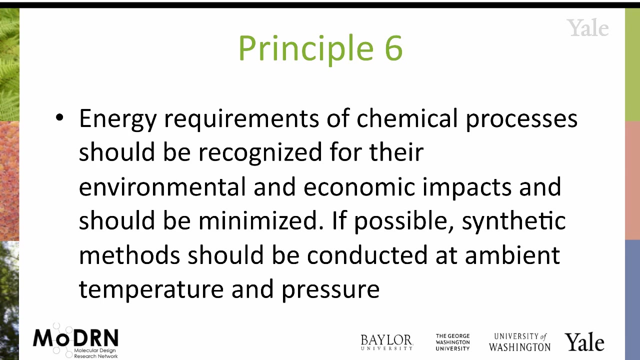 used in the manufacturing process. so we can't underestimate this, so that they there are ways to not only come up with alternative solvents and other auxiliaries that are less toxic, but also ways to eliminate them completely. principle six: energy. energy and the nature of its energy needs to be understood. how much embedded energy is? 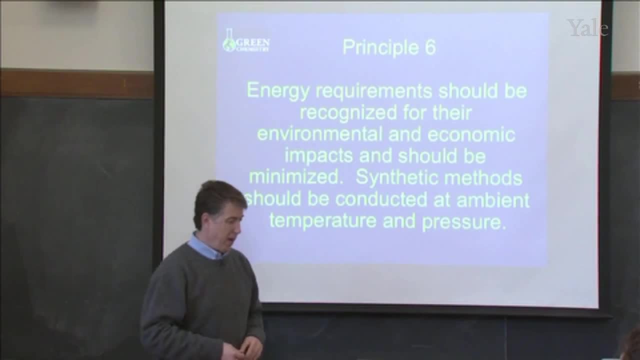 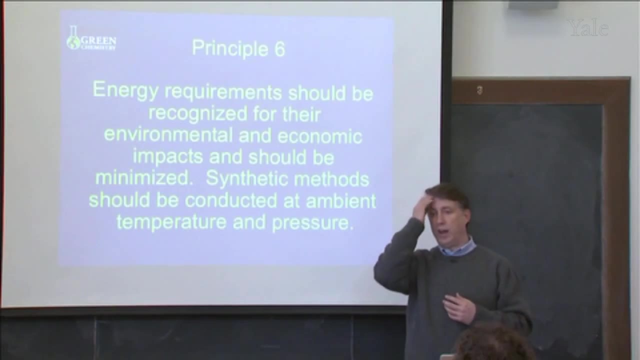 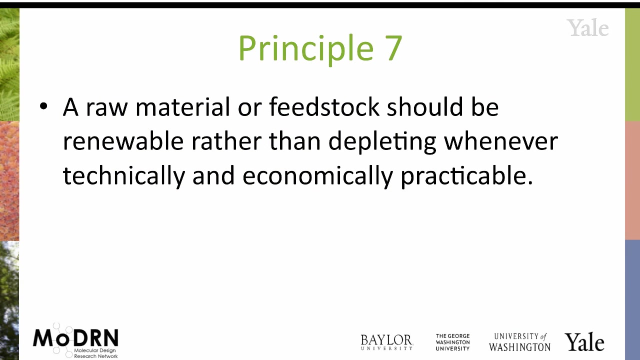 going into the harvesting or mining. how much of how much energy is going into the manufacturer, the separations, the isolation, the purifications and the nature of that energy? is it renewable, is it? is it fossil? is it depleting? principle seven: a raw material. this is our feedstocks question should be: 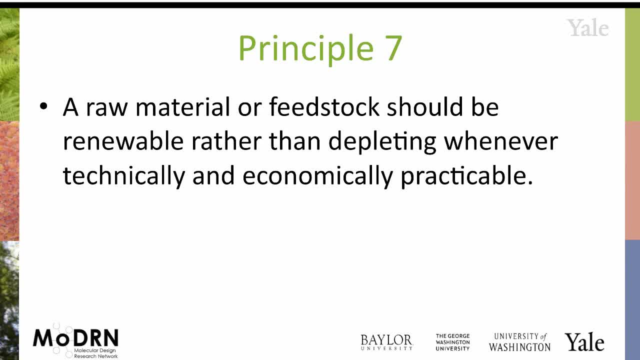 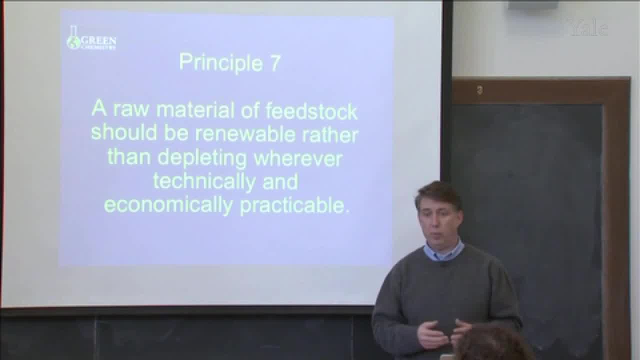 renewable rather than depleting, rather than technically and economically practicable. renewable, renewable- what kind of timeframe oils renewable? they just need a few million years, so not on a geologic timeframe, we're talking in a human timescale. if you're, you're not able to renew this on your, your materials. 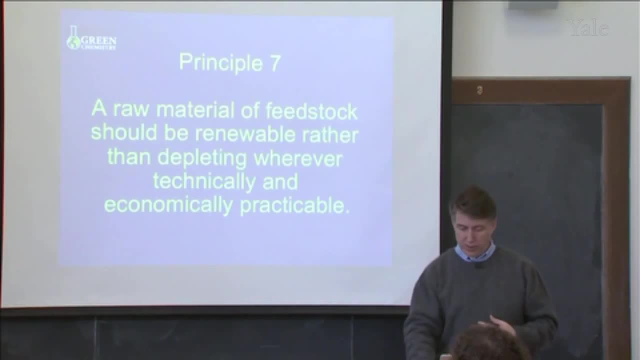 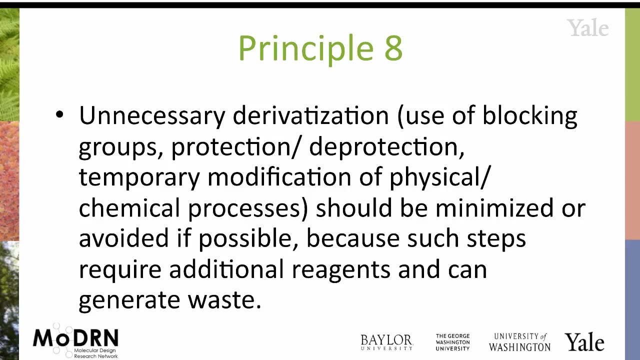 on a time frame. then there you're, definitionally depleting. principle eight: this is more subtle. it's a. actually, in order to get from a to B, many times you have to go through other ways to get from a to B to a different way, and that's a. 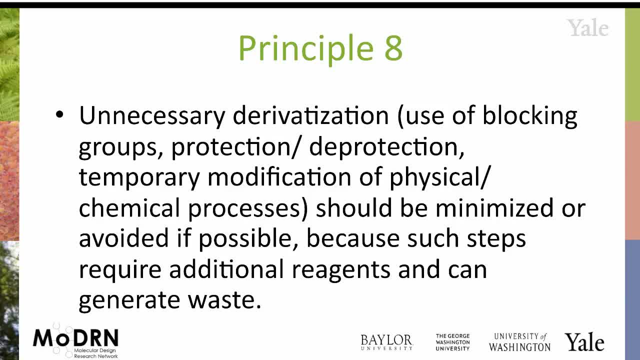 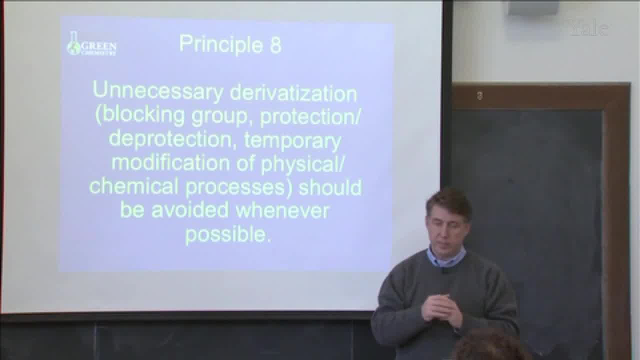 A double prime, A prime, A double prime, A triple prime, and you transform it on your way to B. That has been the way for 100 years: coming up with ways of, instead of going through all of those other steps that generate all kinds of ways. 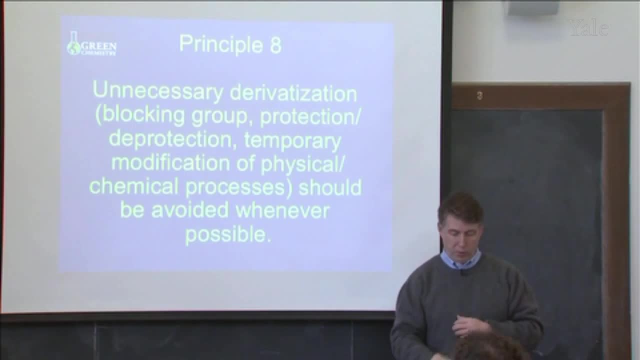 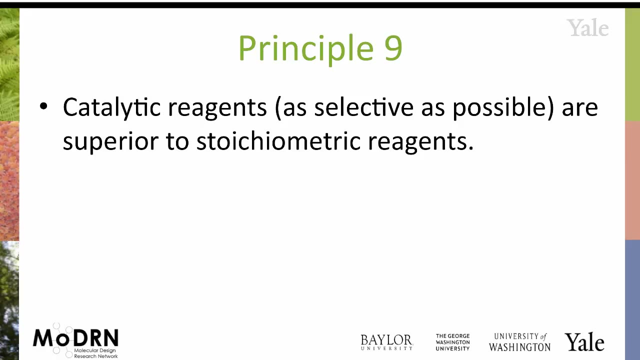 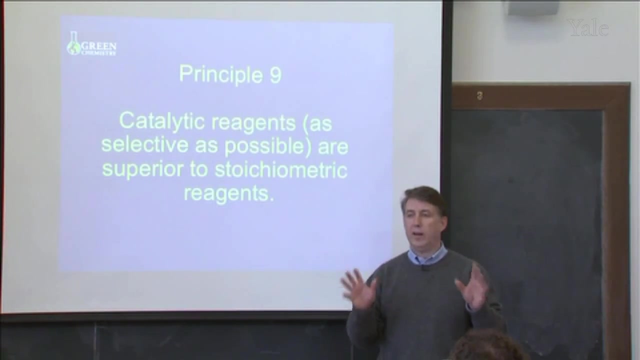 use all kinds of material. instead, come up with ways, the way you can eliminate these steps. Catalysis: we are going to devote a whole focus to catalysis. We'll be discussing what catalysis is and the spoiler alert: catalysis allows you. 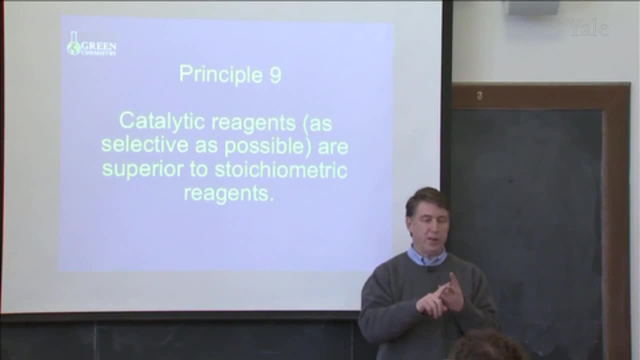 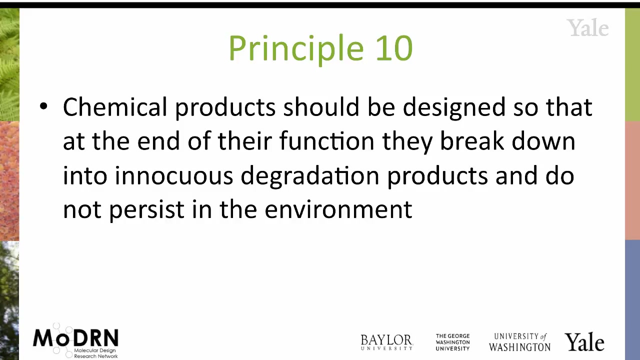 to make product with less energy, less material, less waste, and there's not a petrochemical, pharmaceutical specialty, chemical company that would be in business today without it. Principle 10, products should be designed so at the end of their function.